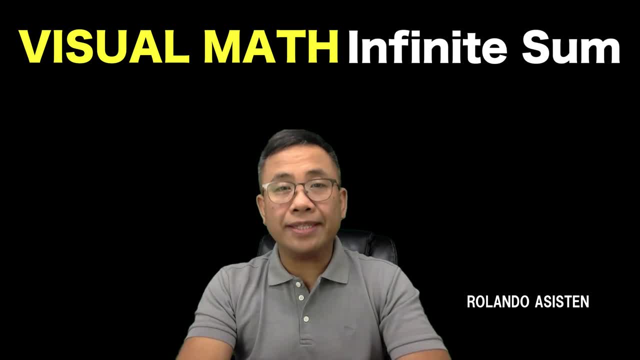 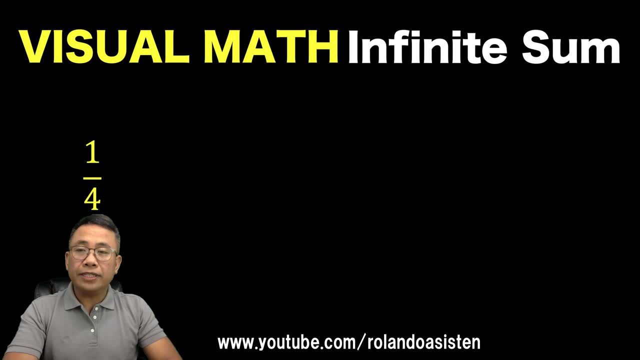 Hi guys, in this lesson I'm going to show you the beauty of mathematics in the visualization of infinite geometric series. Let's begin our lesson. Let's say we are given 1 4th plus 1 4th to the second, plus 1 4th to the third, plus 1 4th to the fourth, until infinity. What is the sum of this? 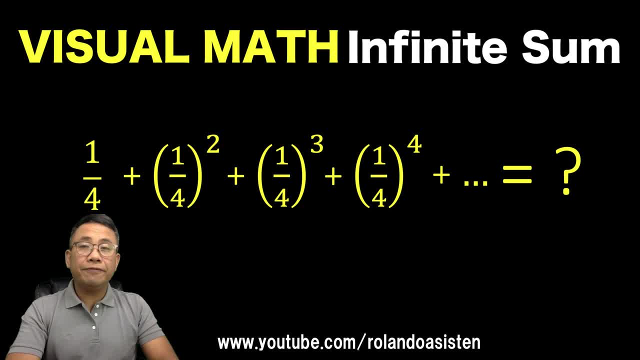 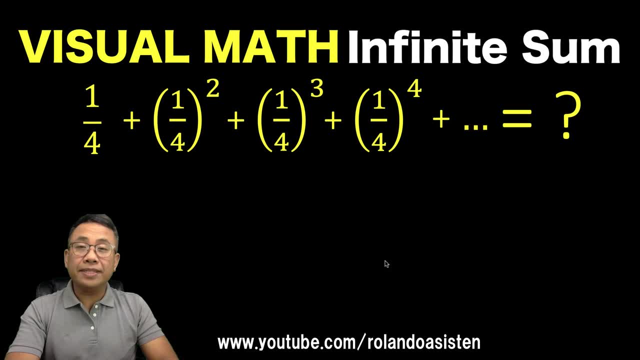 infinite geometric series. Let me show you two methods. The first one is using visualization and the second one is using a formula. Now, this kind of repetitive sum can be written in a shortcut method. this way: It's the sum of 1- 4th raised to n, where our n starts from exponent 1. 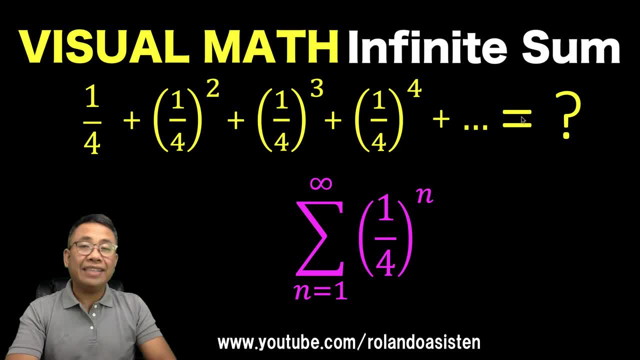 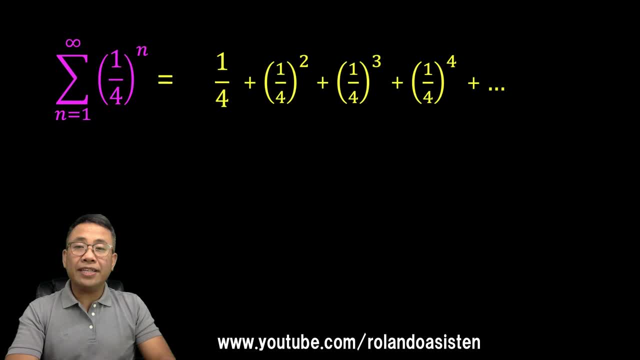 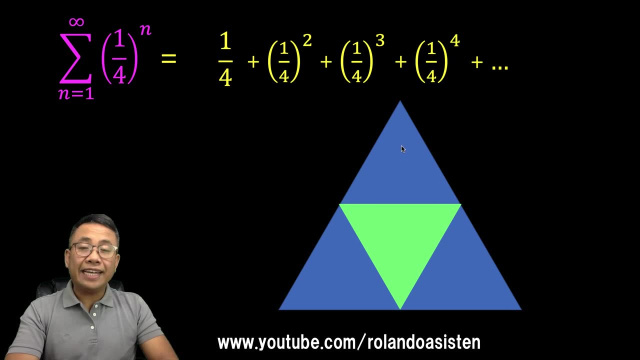 exponent 2, exponent 3, exponent 4, until infinity. So what is the sum of this infinite geometric series? Let's begin by visualizing first our first add-on here: 1, 4th. If you have this blue equilateral triangle and divide that triangle into four equal parts, we have 1, 2, 3, 4. 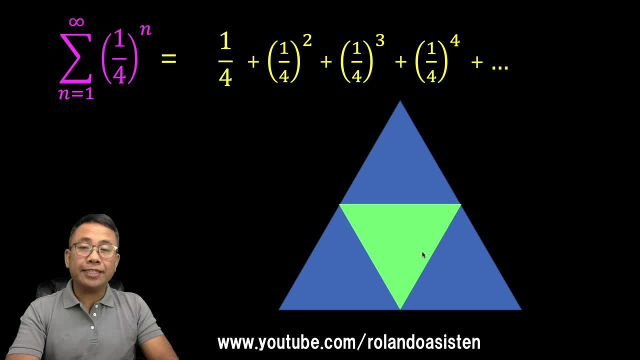 and we take one part out of those four parts, then the area of this green triangle is this: 1 4th. Then take this upper 1 4th and get 1 4th of 1 4th in order to get 1 4th squared. Then take again. 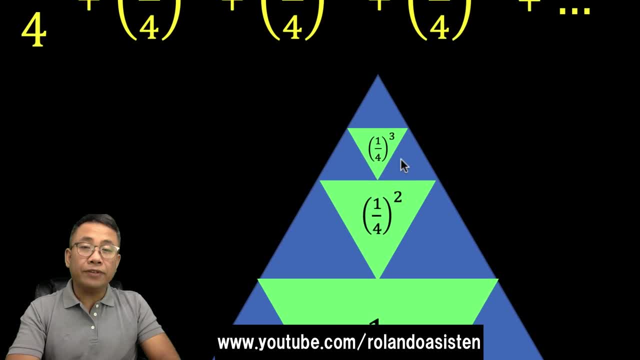 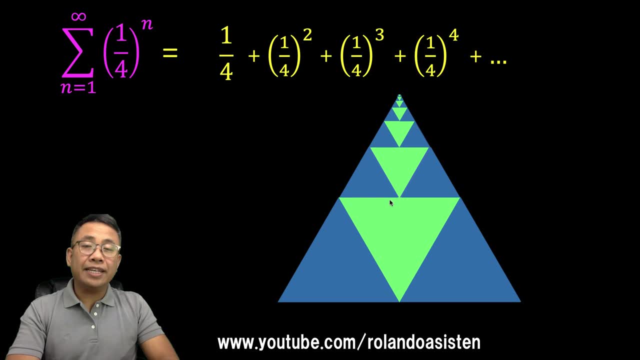 1 4th of this, 1 4th of this, 1 4th- to get 1 4th to the third and continue the pattern repetitively until infinity. Now, from this visualization, it is clear that there is a limiting value for the area of this. 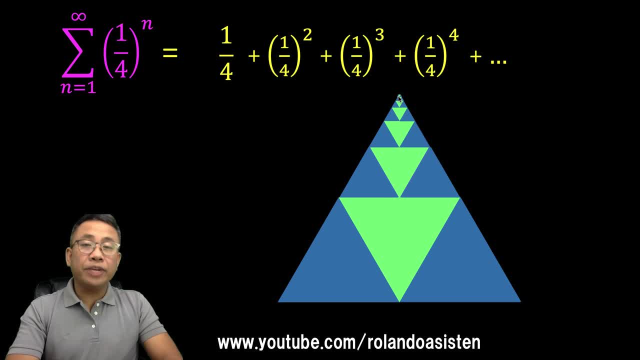 green triangles. In other words, this series will converge to nothingness because eventually the area of this green triangles would become extremely small, converging to a limiting value of zero. Now, how can we use this visualization to find the sum of this series? So look closely, as. 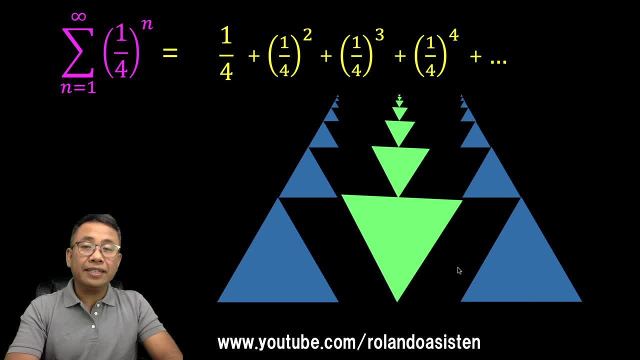 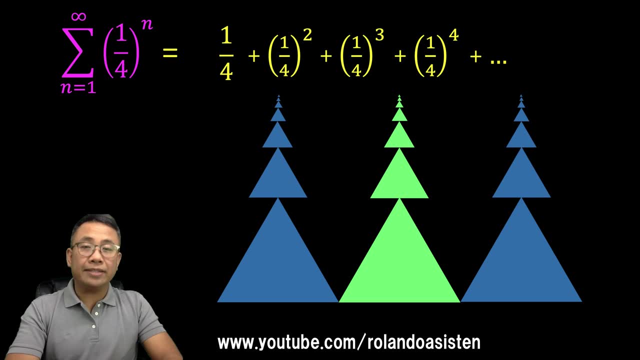 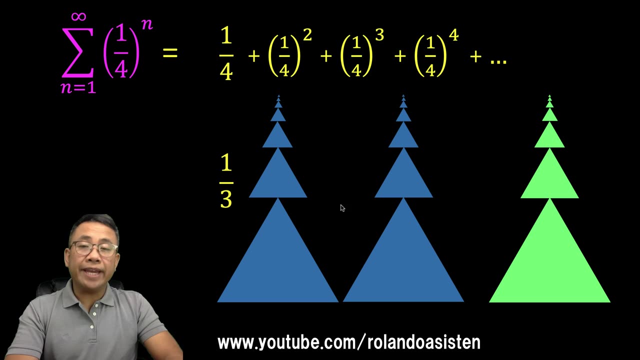 I separate these columns of triangles. Let's reorient the green triangles and let's rearrange the blue columns of triangles. Then let's swap places of these green and blue triangles. The first column of blue triangles represent one third of the area. This is another one third and this is another one third Notice.